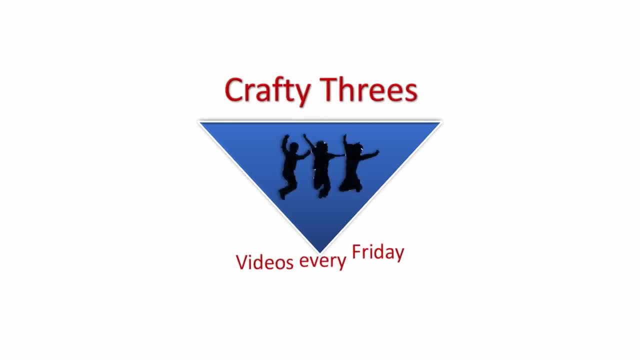 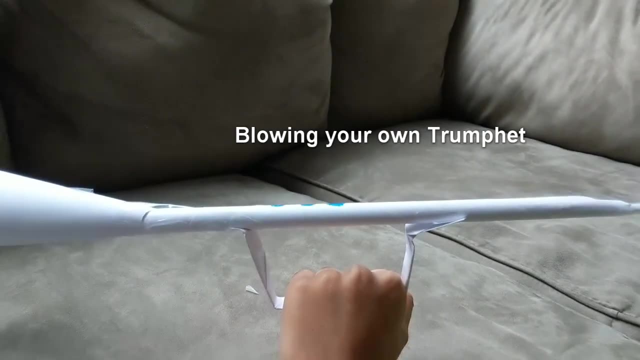 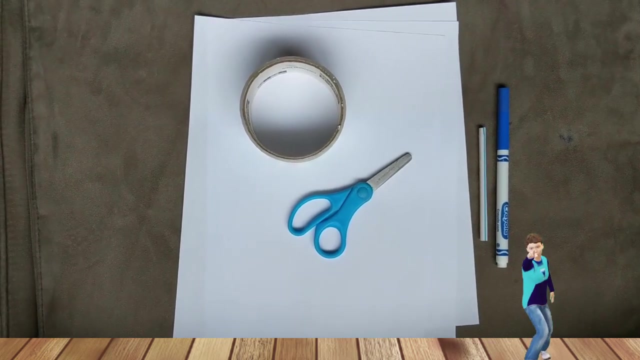 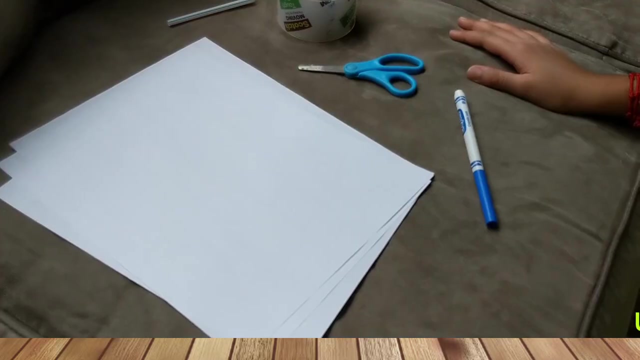 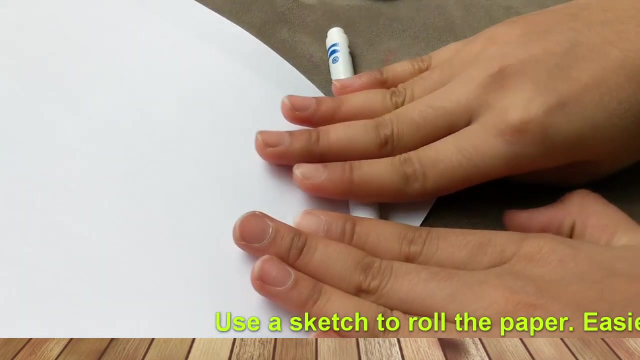 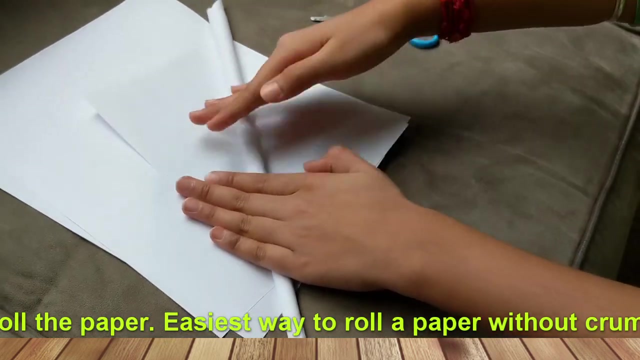 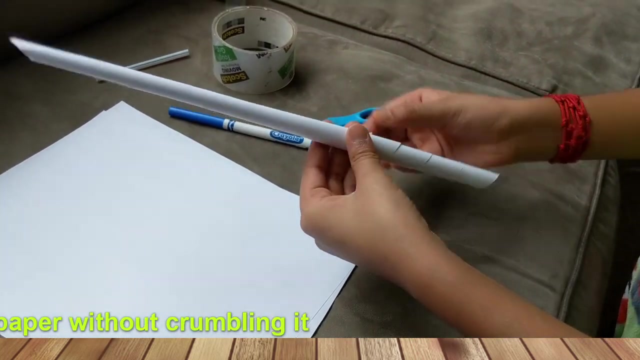 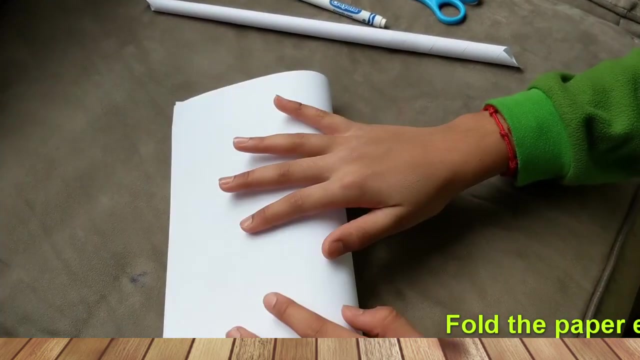 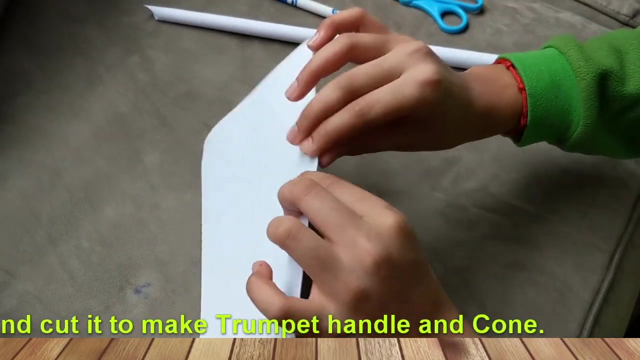 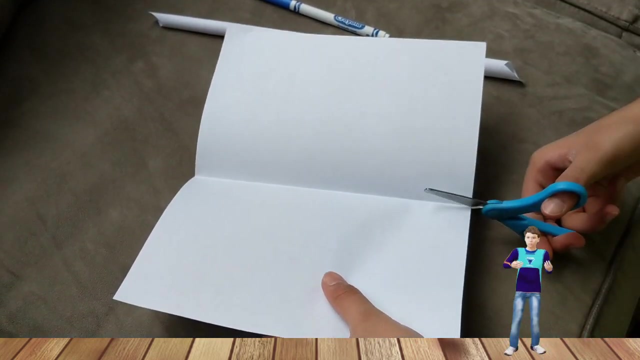 Hi, I am your Crafty One. Come on, let's blow the trumpets, Start music. Hi, I am your Crafty One. Come on, let's blow the trumpets, Start music. Hey, do you know the meaning of the phrase blowing your own trumpet? 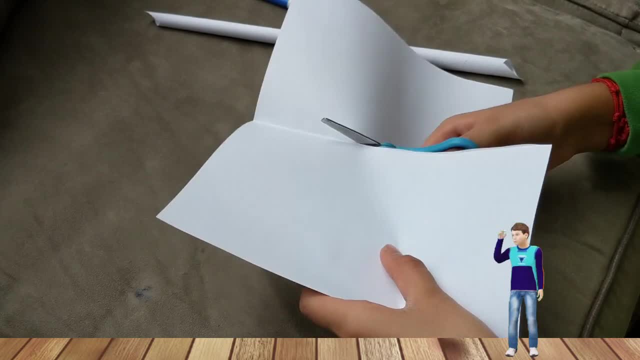 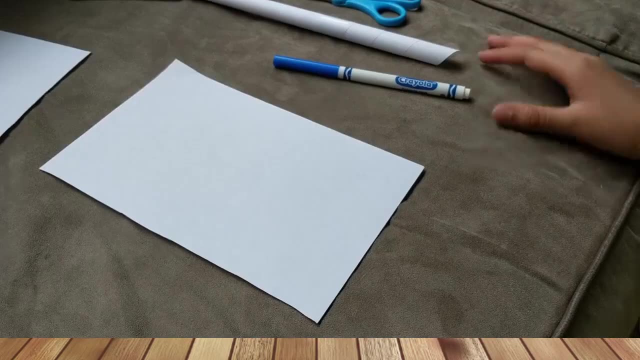 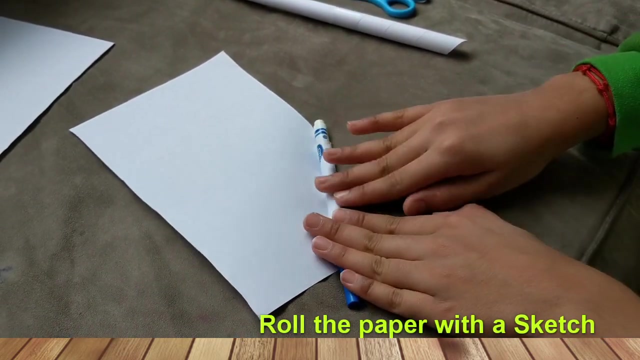 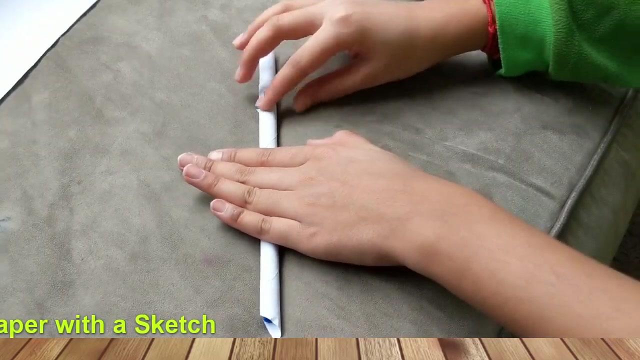 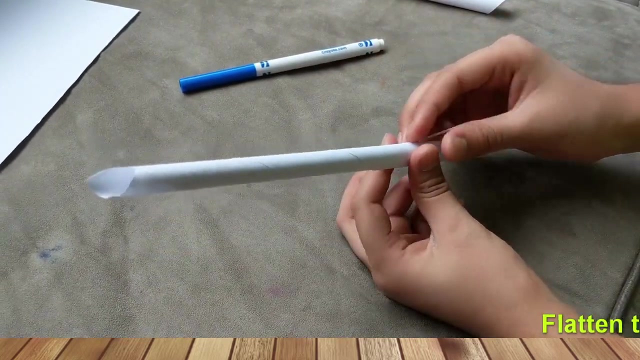 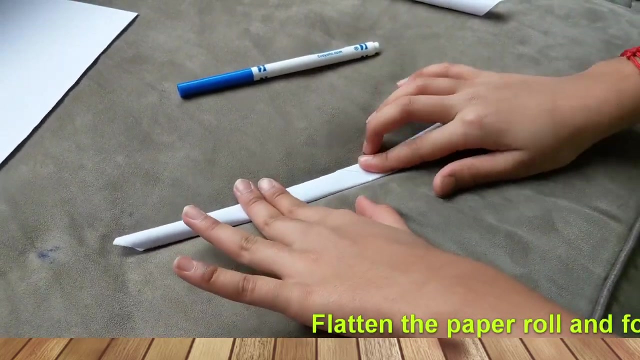 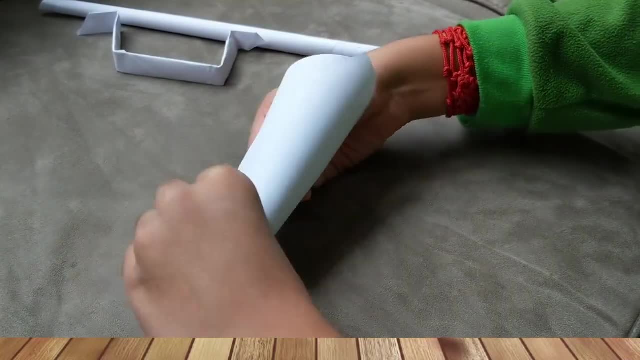 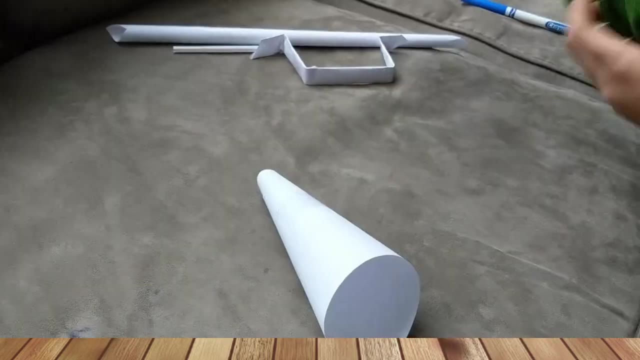 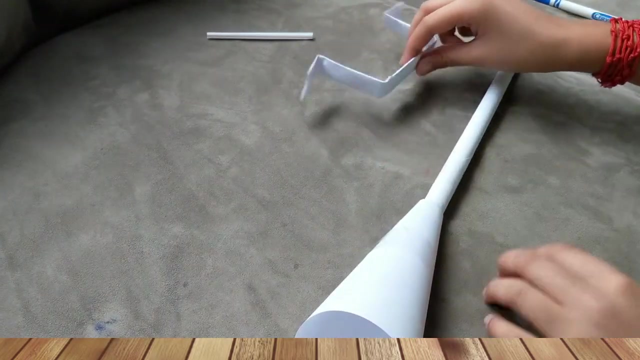 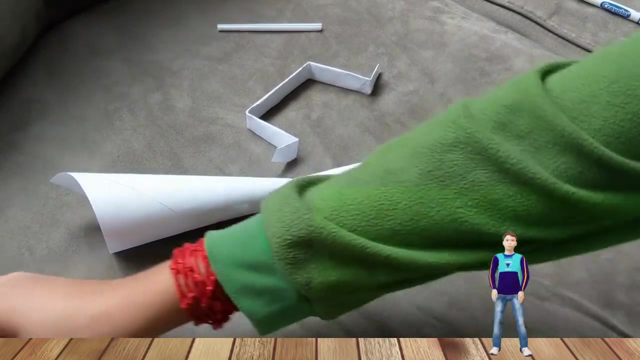 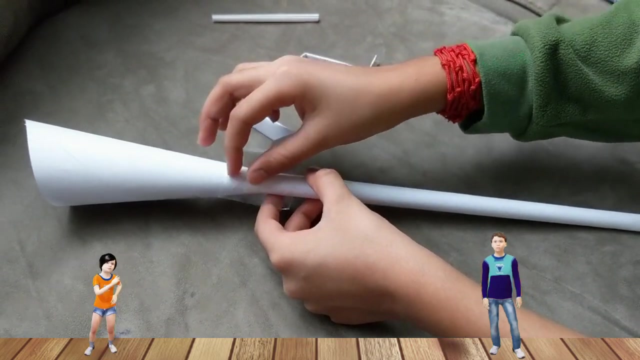 Music. I'll give a demo on the phrase. Watch out, Hi, I am your Crafty Two. Hope you saw my video. Kids, Kids, Kids, Kids, Kids, Kids Time learning world block craft. If you missed it, please click the card above. 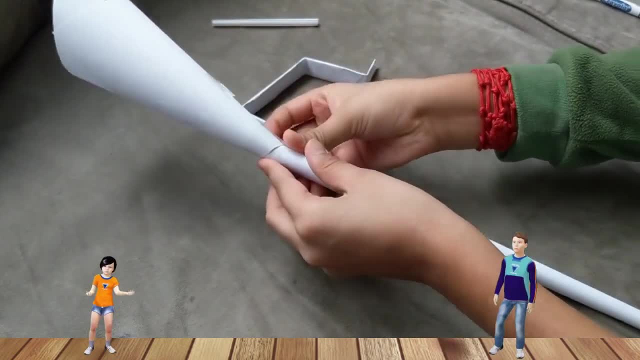 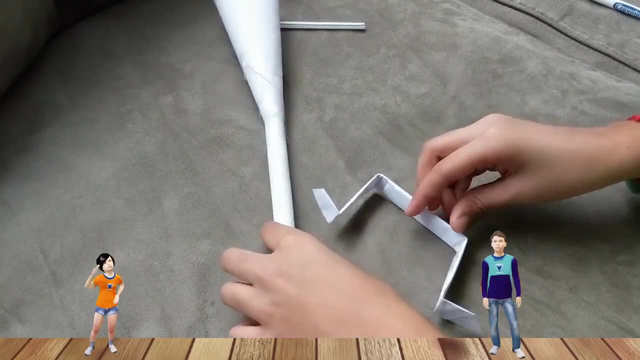 I also do magic tricks. Check the card above to see it. I know salsa dancing. Please click the card above to see our celebration of first month in YouTube. I dance better than Crafty1 and Crafty3.. This is Crafty2's demo. 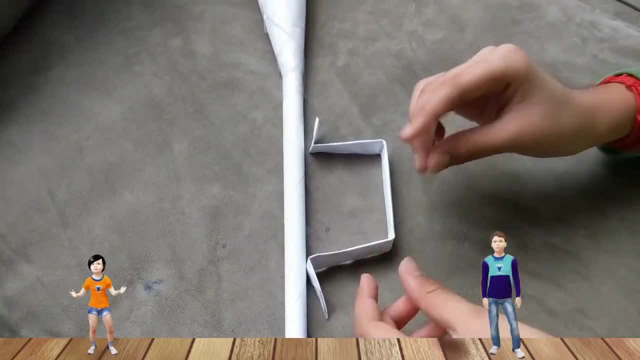 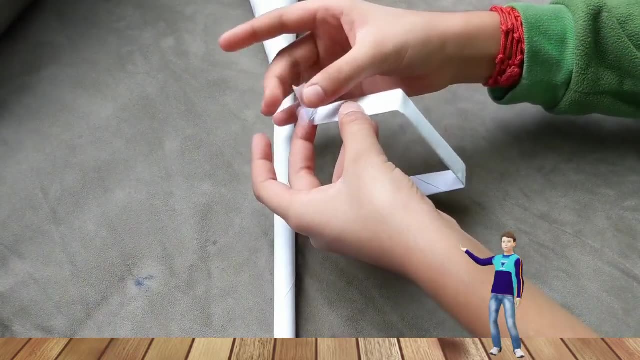 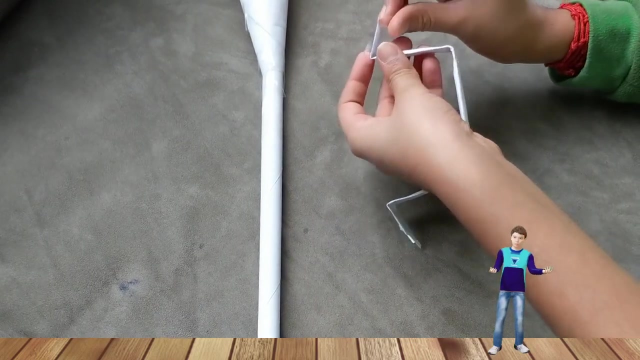 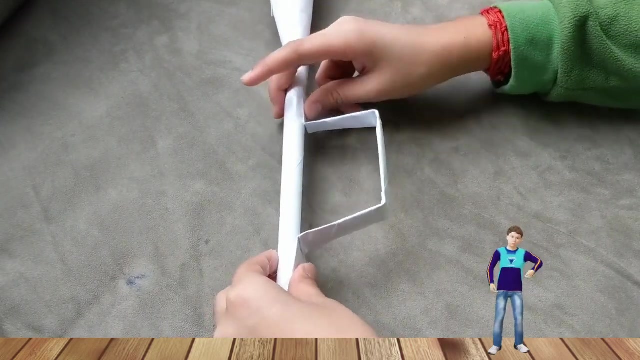 What Am I doing? a demo for your face? Oh, no, To talk about oneself or one's achievement, especially in a way that shows that one is proud or too proud. Yes, we had a good demo Time for a math question. If 1 is equal to 5, 2 is equal to 10, 3 is equal to 15 and 4 is equal to 20,, what is 5 equal to? 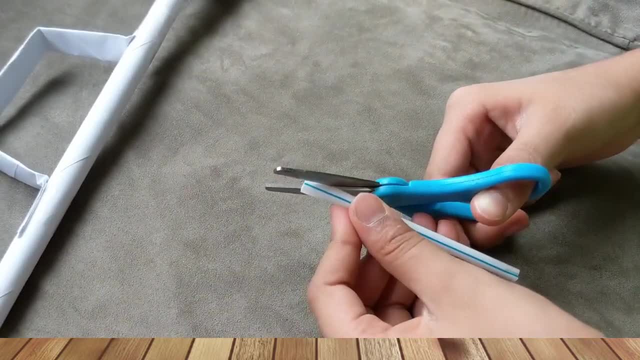 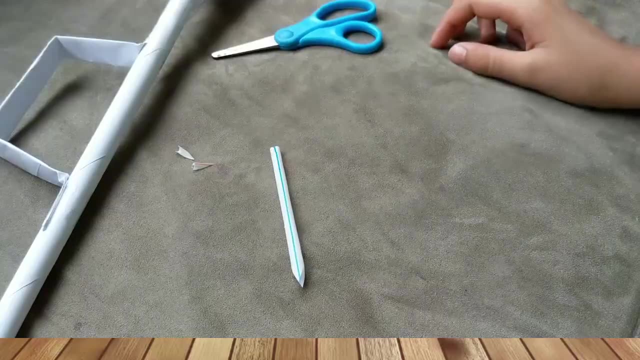 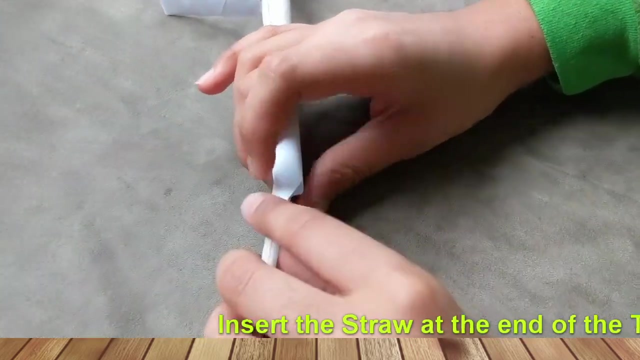 I will tell you in a minute. If 1 equals to 7, 3 equals to 10, 5 equals to 3, what is 5 equal to 15 and 6 equals to 10? Math. I don't know how to answer this question, but I think it is hard to answer because it is important. 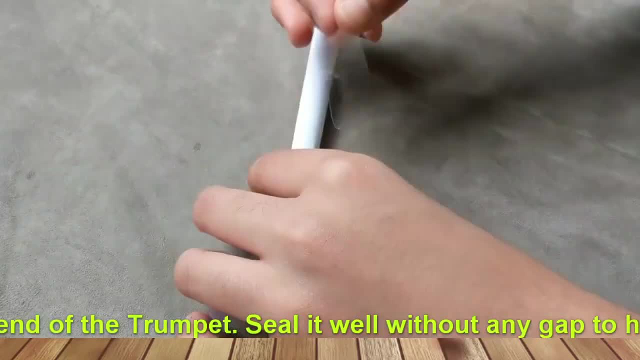 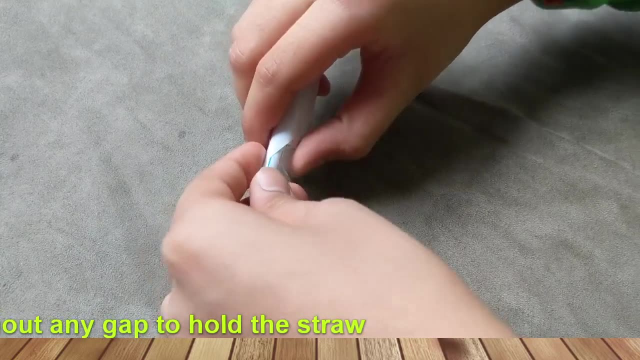 The answer is simple. Do you know how to solve this question? Yes, Let's try. 1 equals to 10 equals to 15.. What is 5 equals to 10?? I don't know, I can't answer it.